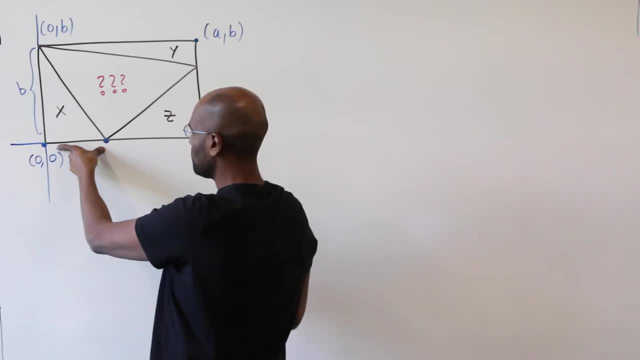 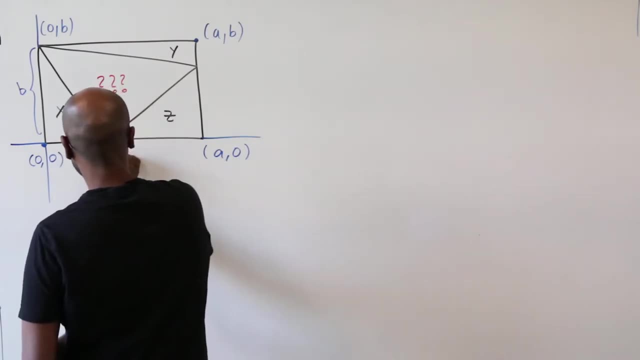 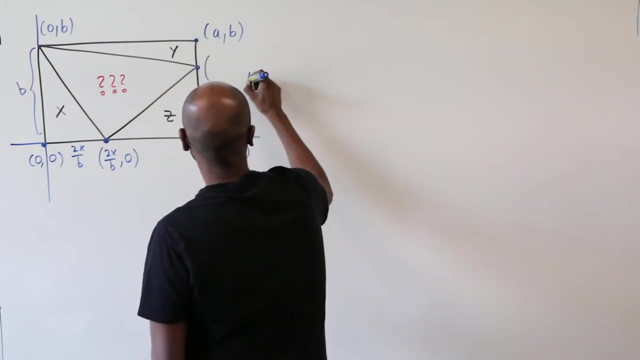 so the product of b and this thing has to be twice x. Consequently, this length is 2x over b, and so the coordinate here is 2x over b and 0.. We can do a similar thing to figure out this coordinate right here. 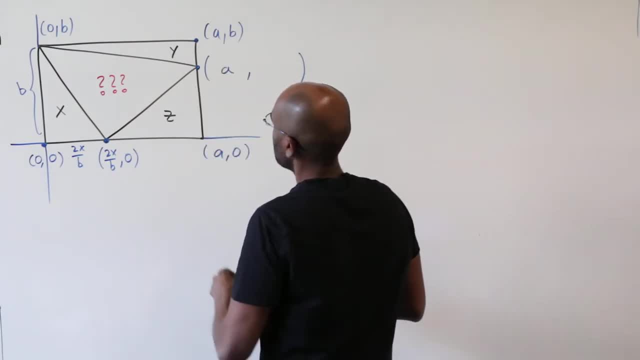 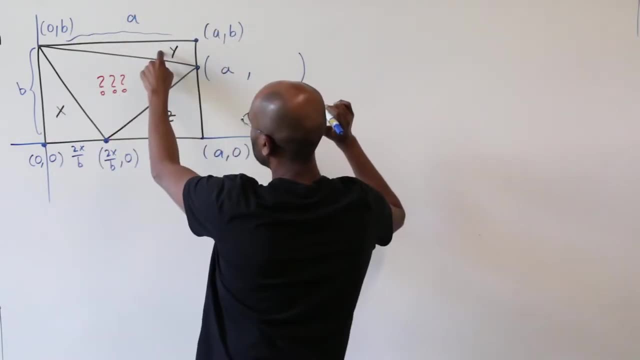 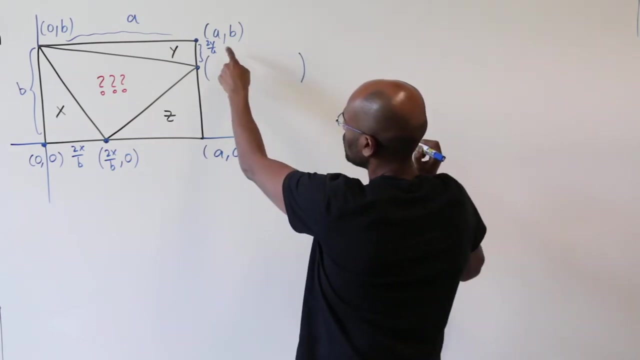 We know that its left coordinate is a. Now the length of this entire side here is a. The area of this right triangle is y, so this length here has to be 2y over a, meaning this coordinate is 2y over a, fewer than b. 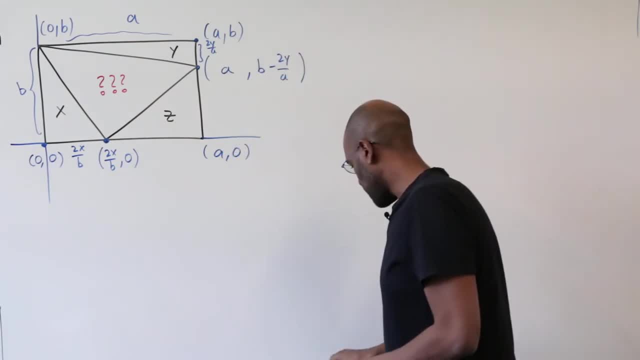 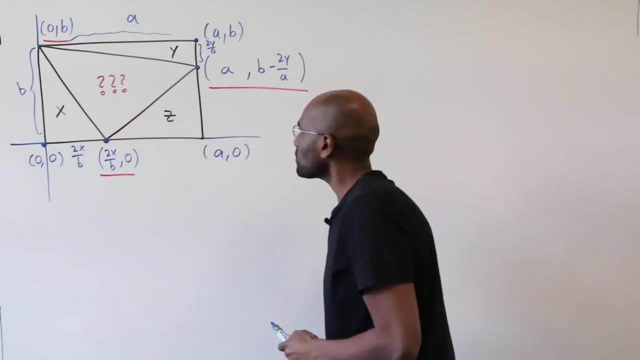 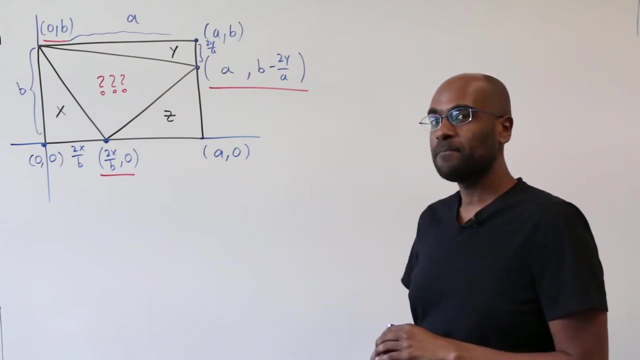 which is b minus 2y over a Great. So now we have the coordinates of the three vertices in question and we're going to express the area of this triangle in terms of these coordinates. Now, the formula to do this is called the shoelace formula. 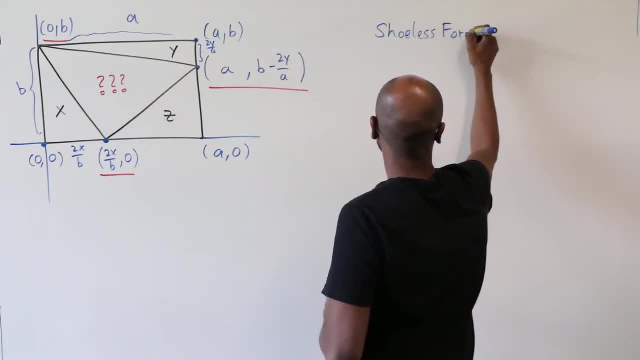 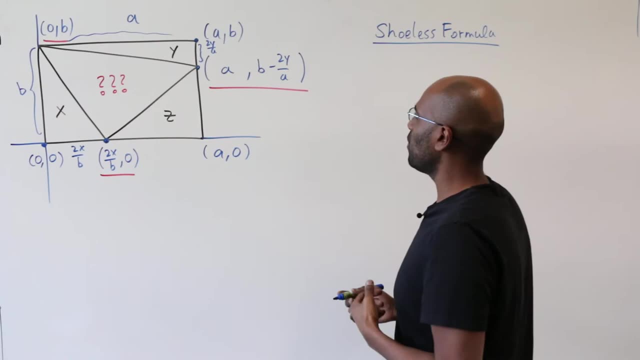 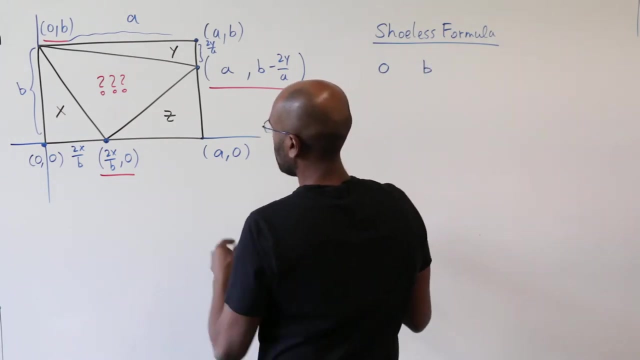 and it's going to look kind of silly, but it actually comes from an interesting place. So I'm going to at least talk about what this formula is and then talk a little bit about where it comes from. So I'll write down the vertices of this triangle in order. 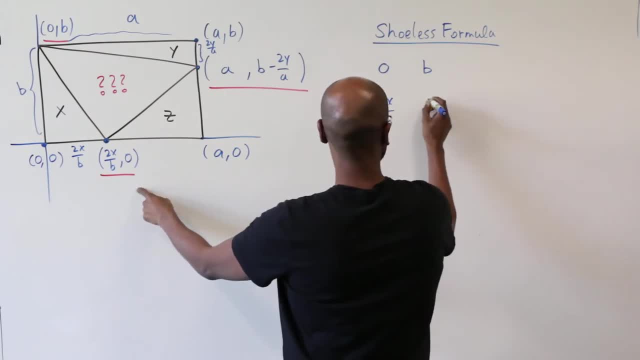 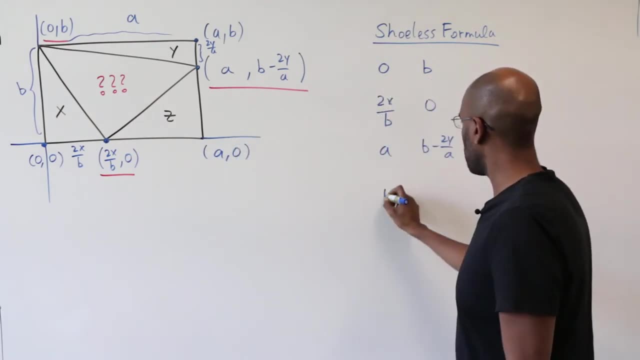 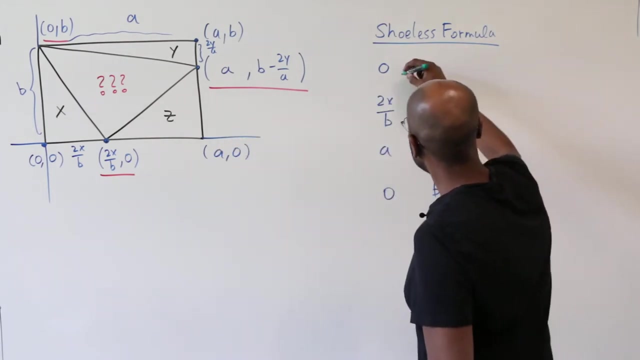 so 0b, 2x, b, 0, and a, b minus 2y over a, And I'm going to rewrite the first coordinate as well. And now I'm going to draw in shoelaces. The shoelaces are going to go downward in one direction. 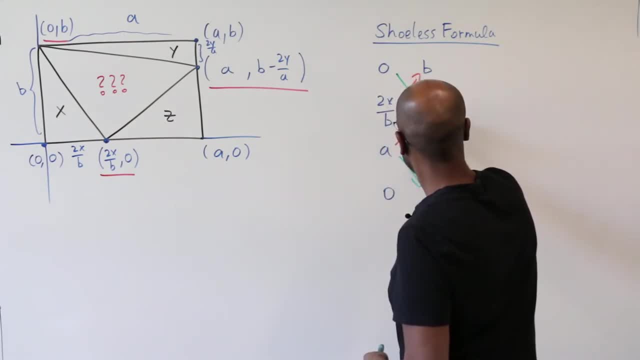 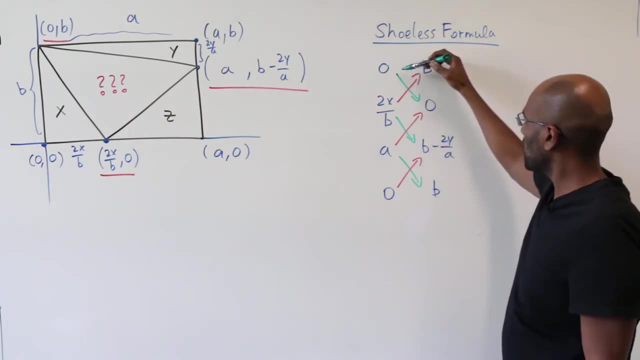 and upward in the other. Now, for each shoelace I'm going to write down the product of the values that that shoelace ties. So here we'll have a 0, and then we'll have 2x over b times the quantity b, minus 2y over a. 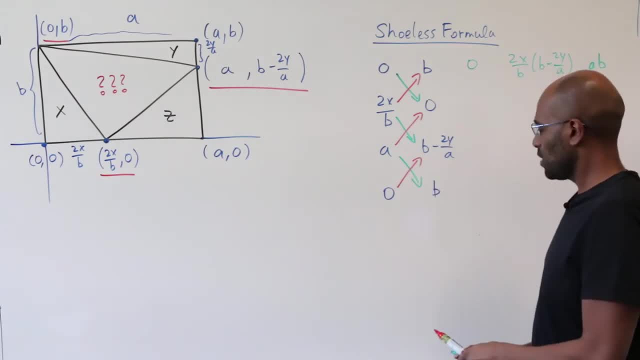 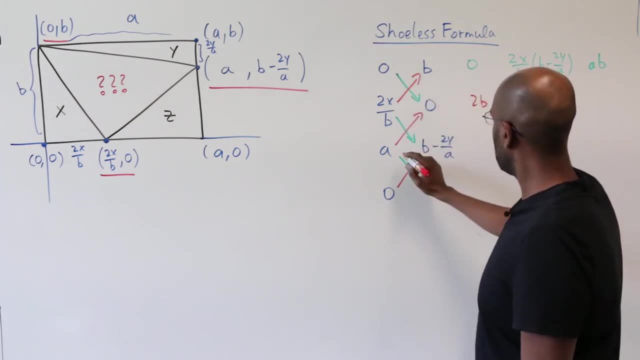 and then, finally, we have ab, Alright, The upward laces. we have 2x over b times b, which is 2b, and then we have a times 0,, which is 0, and 0 times another quantity, which is 0.. 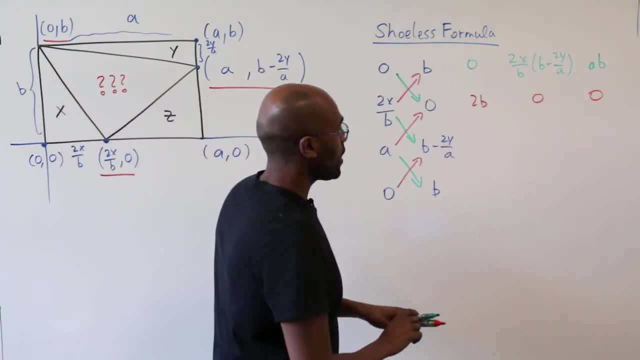 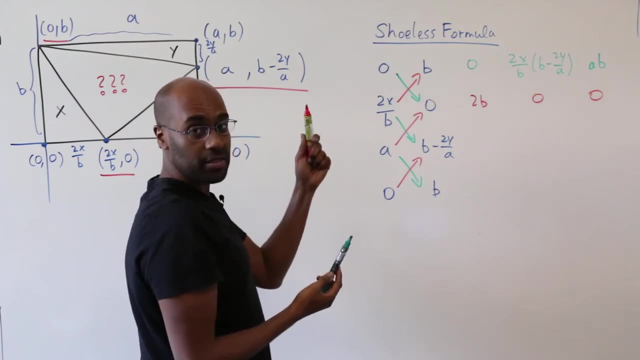 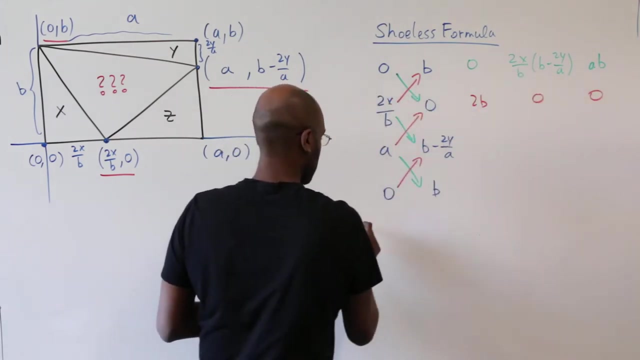 So what the shoelace formula states is that the area of a triangle is the sum of the values in the green laces minus the sum of the values of the red ones. So in this case we'll add up everything in green. If we distribute here, we'll get 2x minus 4xy over ab. 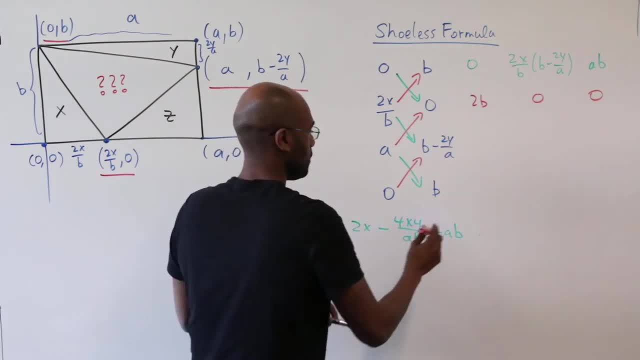 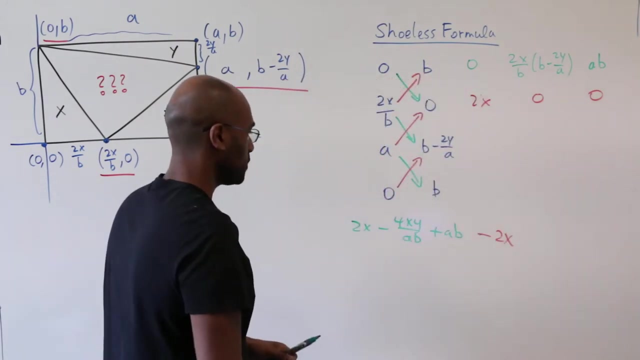 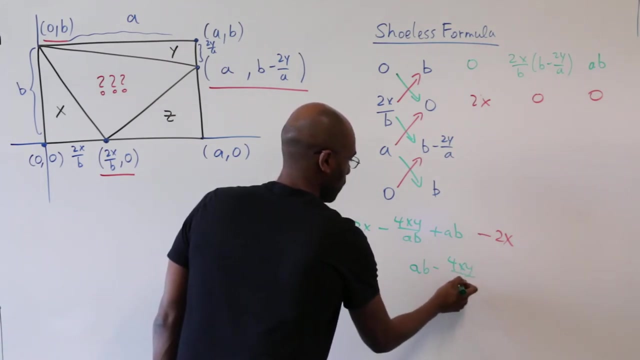 plus ab, and then we'll subtract everything in red, which is 2, should be 2x. actually, This is 2x over b times b, so this is 2x, Okay. so if you simplify that, we get that the area is ab minus 4xy over ab. 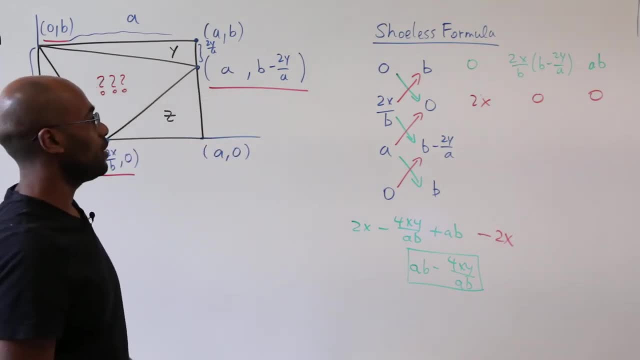 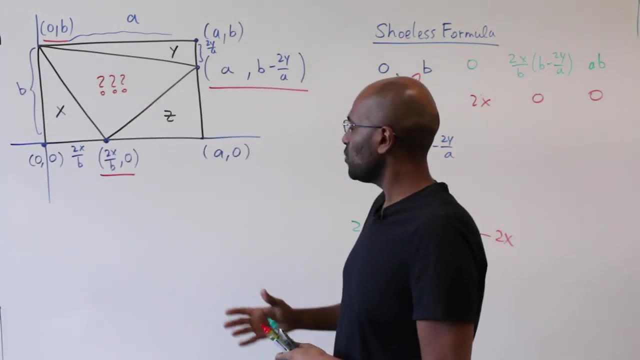 Okay, A couple of comments about this. So, first of all, this seems like a funny formula. It's actually a useful formula. If you have a problem where you don't necessarily know what's going on with the triangle, you can coordinate. and once you find the coordinates, 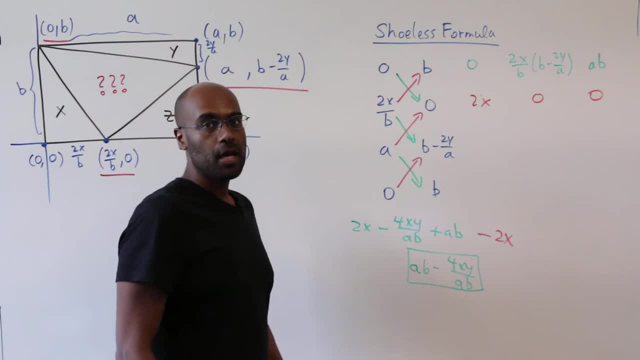 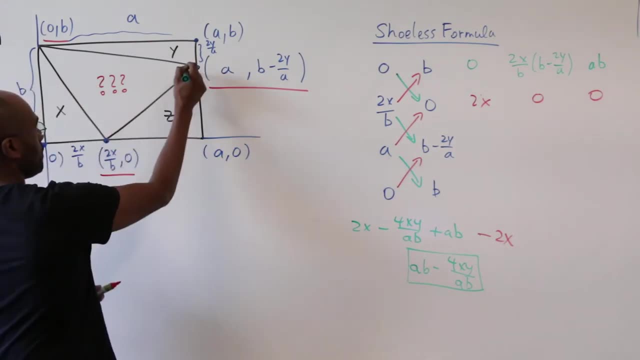 use the formula to find out the area A little bit about where it comes from. This actually is an expression for the cross product of the vectors emanating from one vertex of your triangle to the other two, And it's also related to determinants. 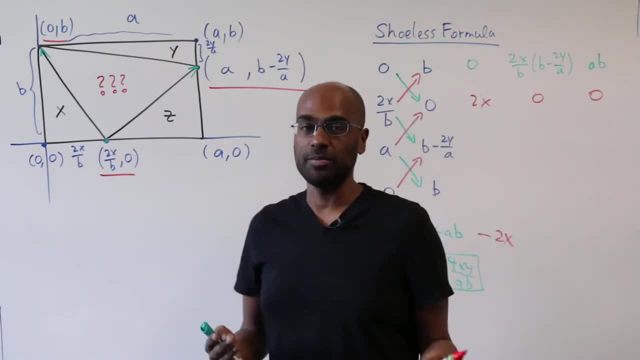 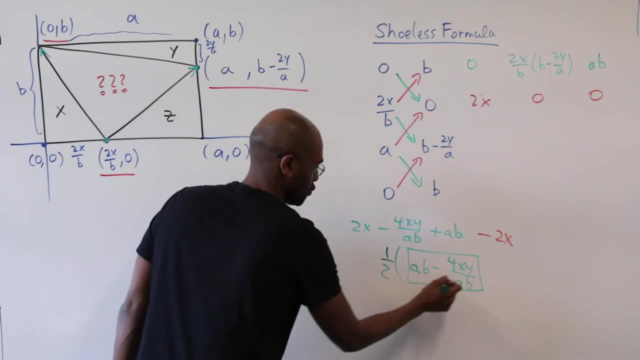 So if you know anything about those two, they both have relationship to area. I should make one additional note here. The area is actually a half of what you get from the shoelace formula, So our area is a half of this quantity, right here. 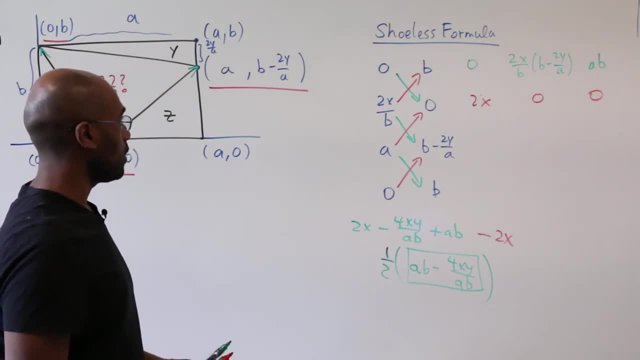 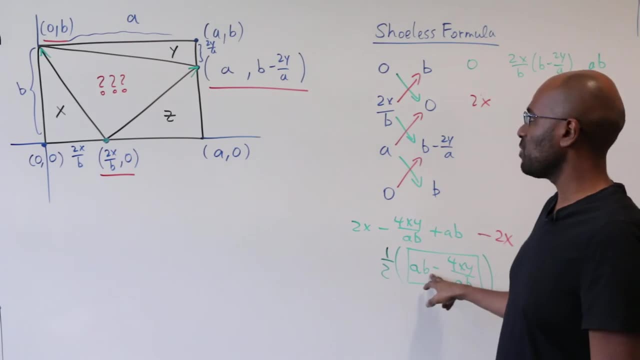 Okay, So this is all good. We have the area in terms of x and y. The only problem is, we also have the area involving variables a and b, which we don't know in terms of our original values x, y and z. 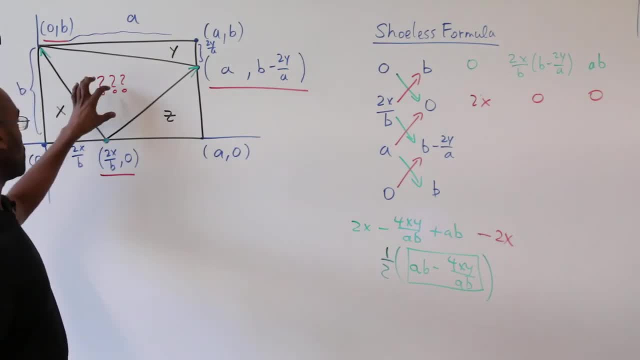 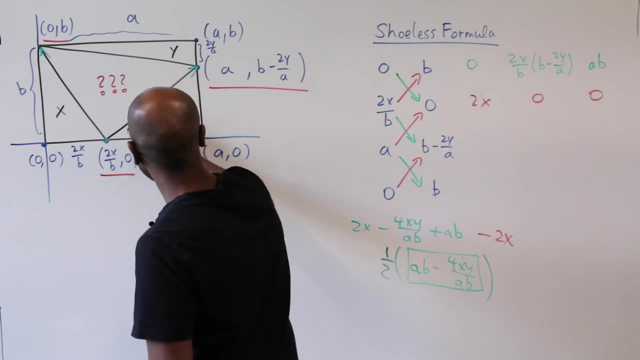 And our goal is to find a formula for the area of this triangle in terms of x, y and z, But we still haven't used all the information here. We haven't done anything with this triangle down here. That's actually something that Presh does in his video. 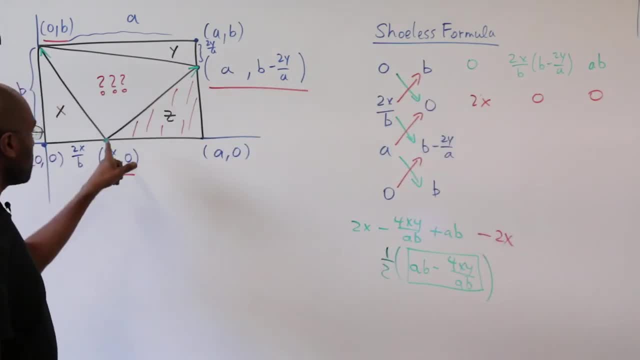 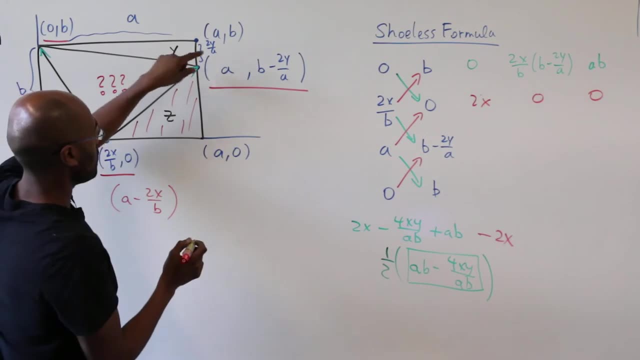 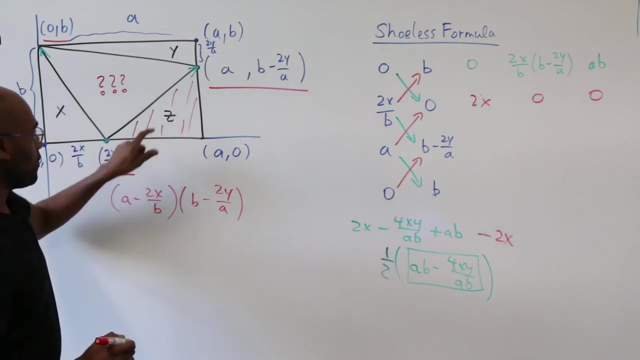 So let's use that to our advantage. The length of this triangle is the quantity a minus 2x over b, And the height here is b minus 2y over a, And that product has to be twice the area of this triangle. 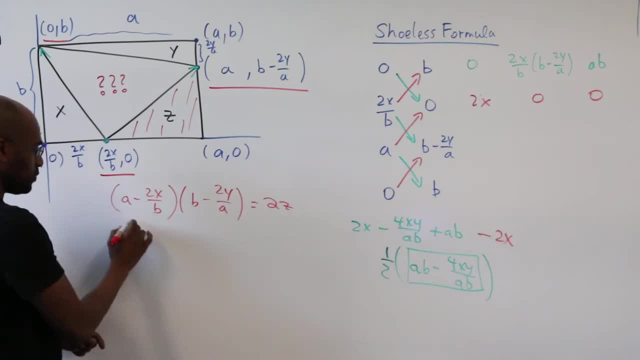 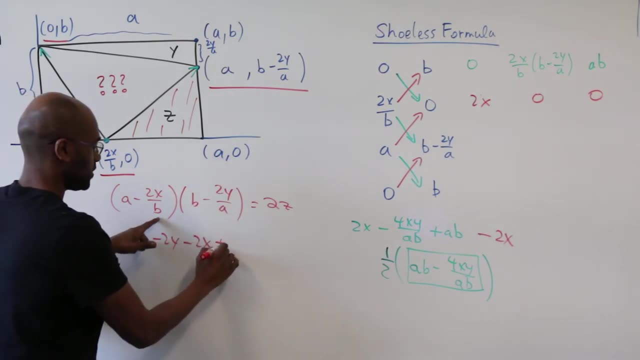 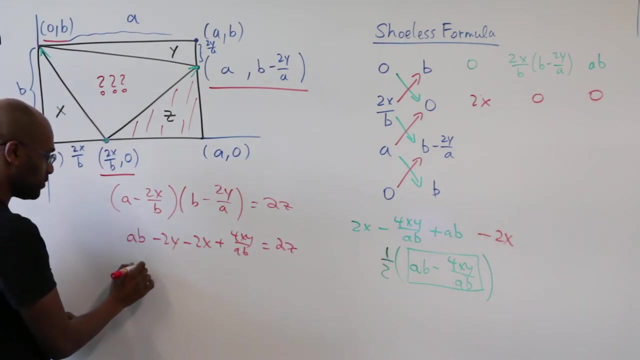 which is 2z. If we expand this, we get ab minus 2y. minus 2x plus 4xy over ab equals twice z, And so at least we have an expression for ab plus 4x, 4xy over ab. 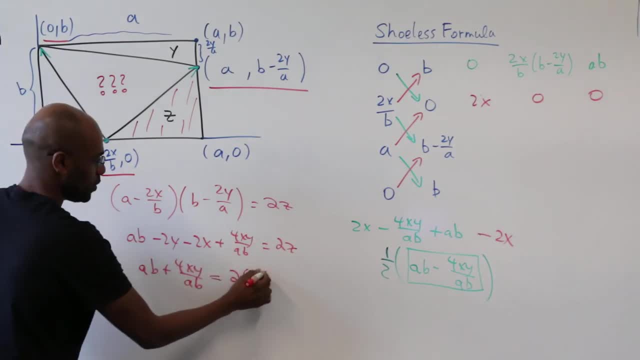 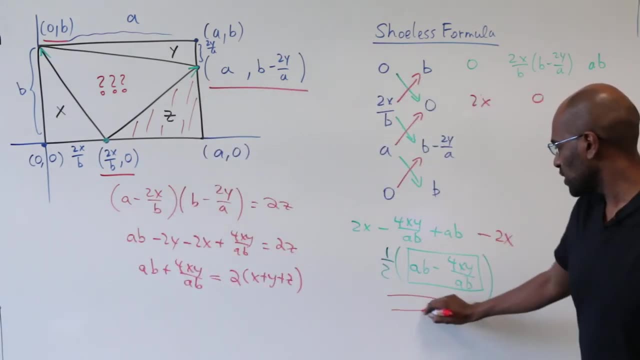 In terms of x, y and z. if we rearrange this, we get 2 times the quantity x plus y plus z. Okay, so here's our area that we're interested in, And here's an expression that we have from our third triangle. 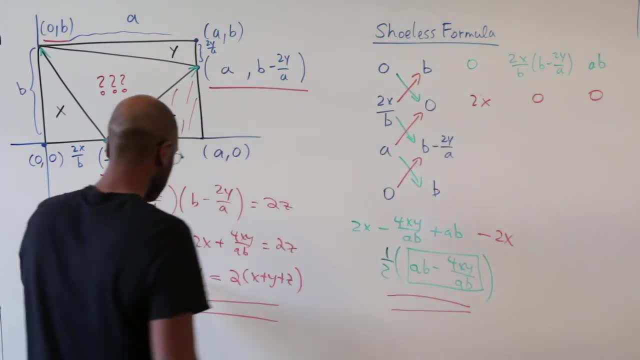 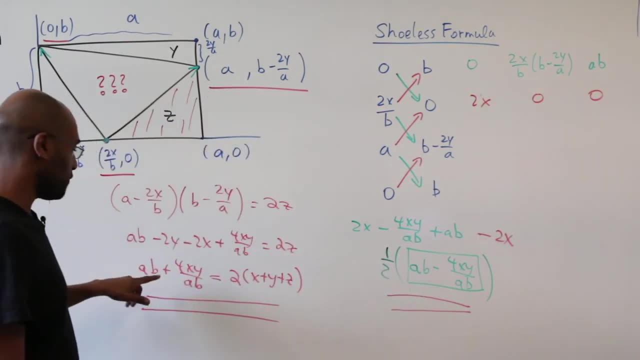 And you notice that the quantity we want looks eerily similar to the one that we have something for. So we're going to now transfer all of this and use algebra to figure out a way to figure out what this quantity is, using the fact that we know this. 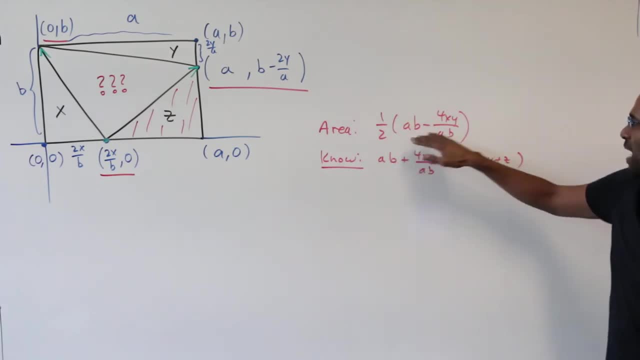 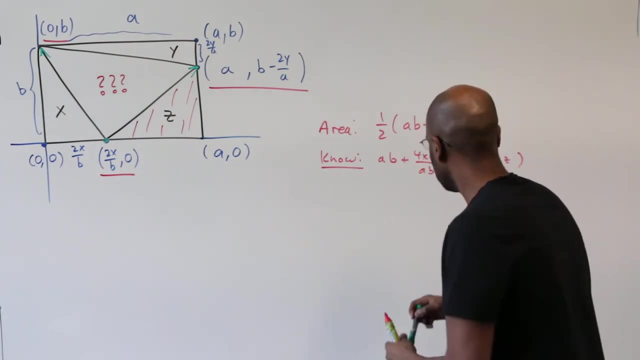 Okay, so the area that we have in question is one half of this quantity And we know that this quantity here is 2 plus x plus y plus z. Now you notice these quantities here and here look quite similar And a way to look at how they're related. 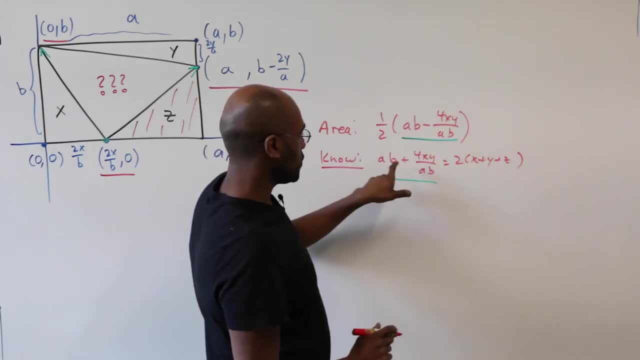 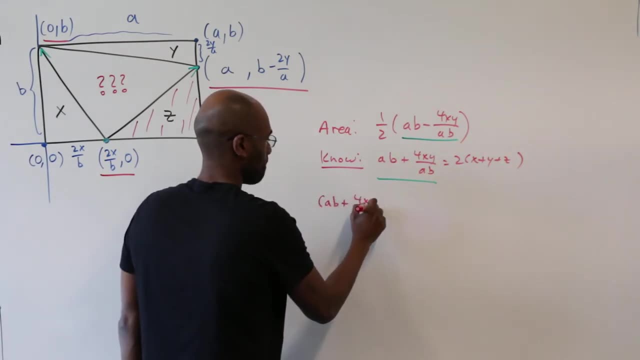 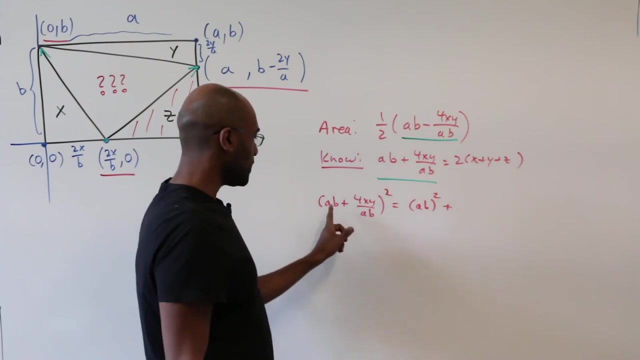 in order to figure out what this value is is by considering squaring both of them. If we square this value here by the distributive property, we get the quantity a, b squared plus twice the product of these two, which is 8xy. 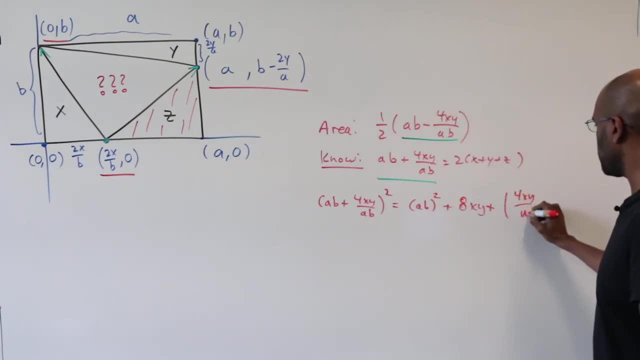 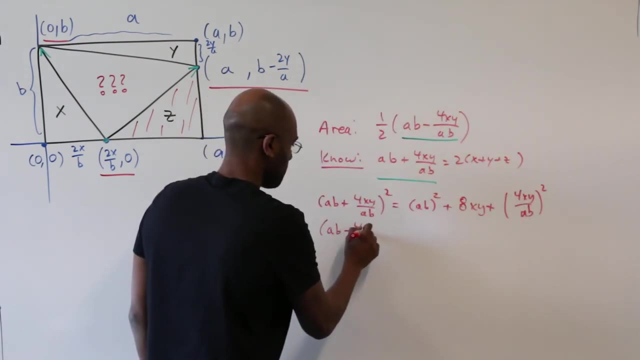 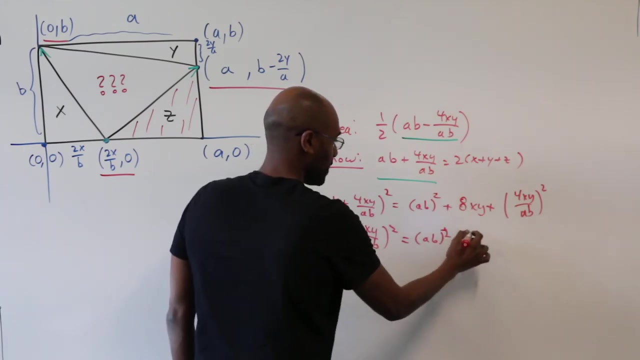 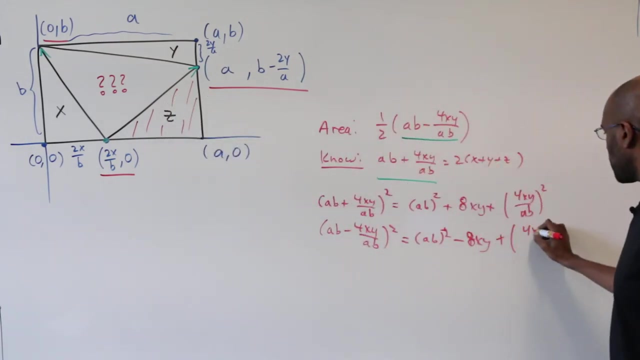 plus the quantity 4xy over a- b all squared. If we instead square the function involved in our area, we get the quantity a- b squared minus 8xy, But then we still have a plus of the quantity 4xy. 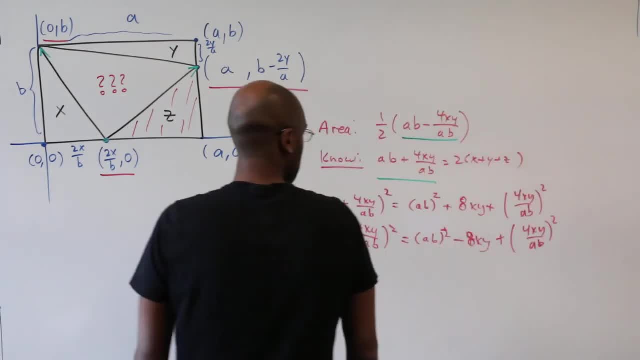 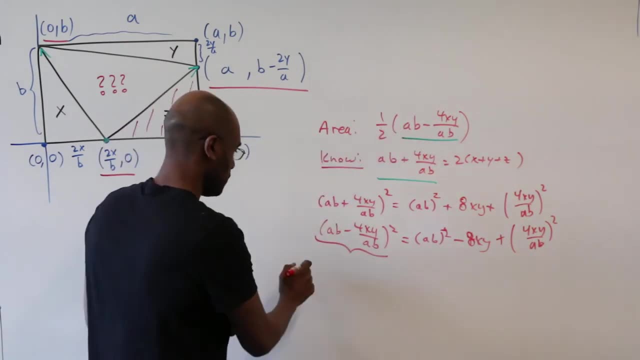 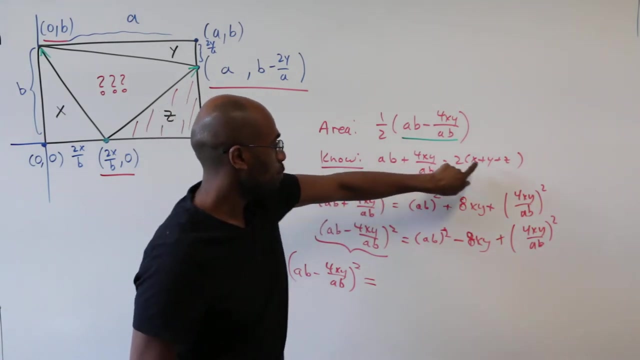 over a, b, all squared. Now, why is this useful? Well, you notice that this quantity, then, which is the quantity related to the quantity we're interested in, is equal to this quantity that we have a value for. this is the square of this thing. 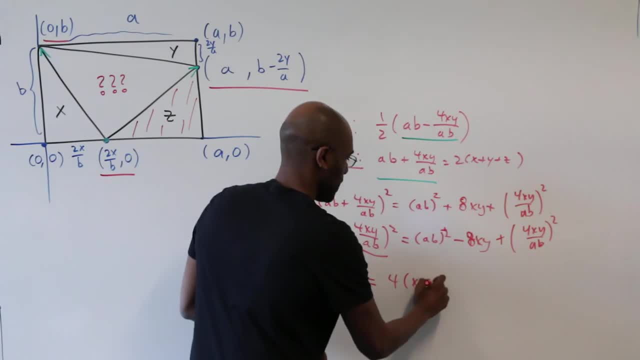 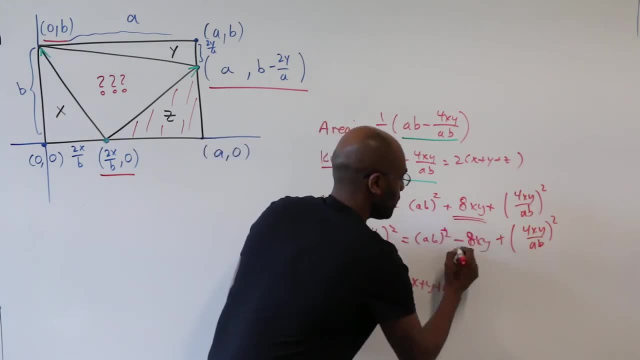 which is the square of this. so it's 4 times x plus y plus z, all squared minus a piece involving only x and y, It's minus 16y. If we take this and subtract 16y, we get this. 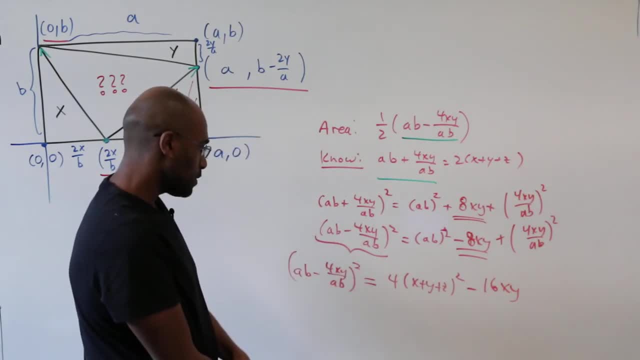 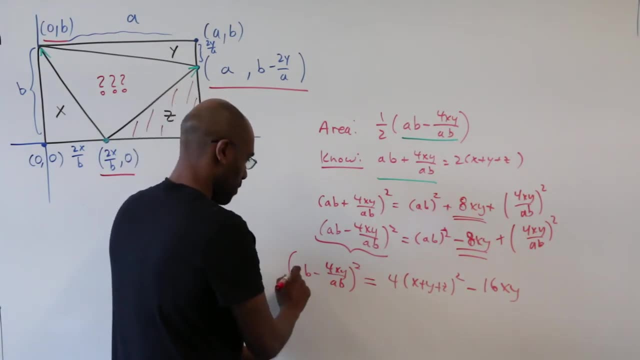 16xy. Okay, great. So now, if we want to figure out what the value of a minus a b, minus 4xy over a b is, we can take square roots. So we'll get the square root of this quantity here. 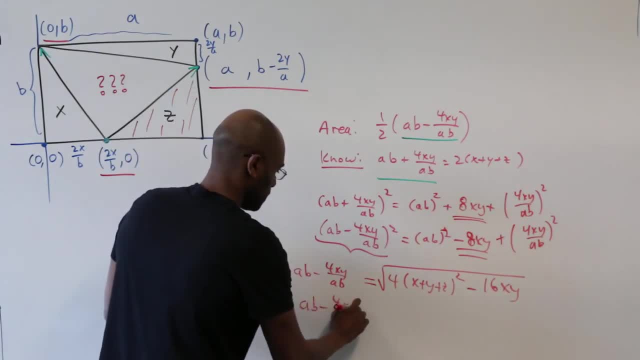 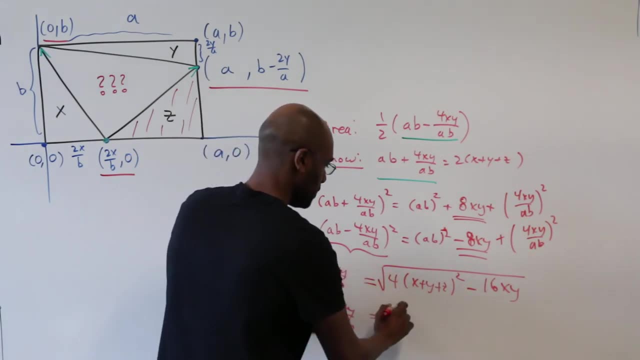 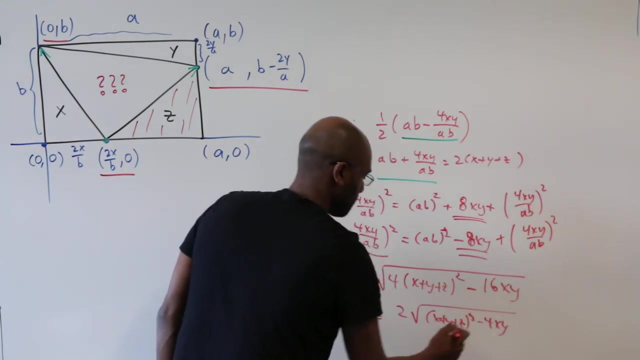 Okay, so subsequently we have that the quantity we're interested in is the square root of this thing. We can factor out a 4, which will come out as a 2. here We'll get 2 times the square root of x plus y plus z, squared minus 4xy. 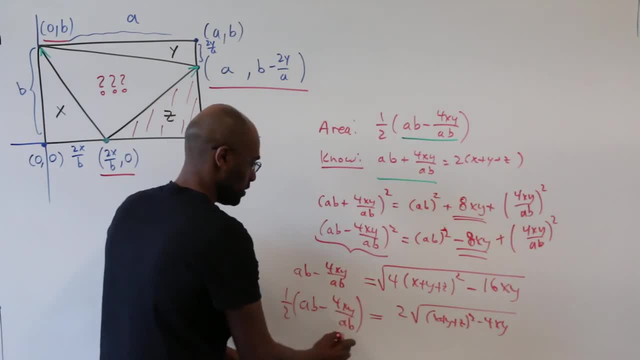 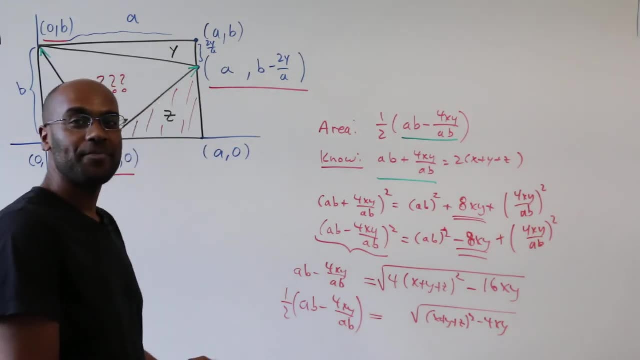 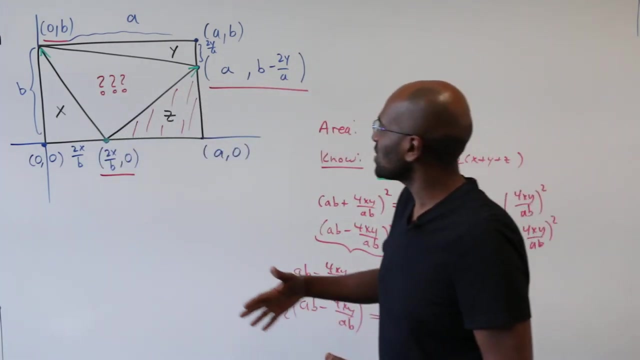 And so the area which is half of this is the square root of the quantity x plus y plus z, squared minus 4xy. Okay, cool. So there's a few more rules to the story here. One is that we wanted the area of a triangle. 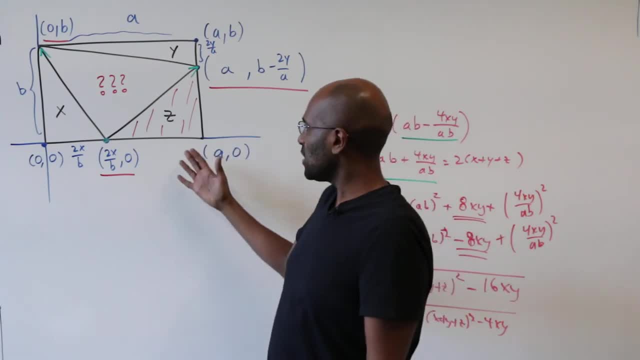 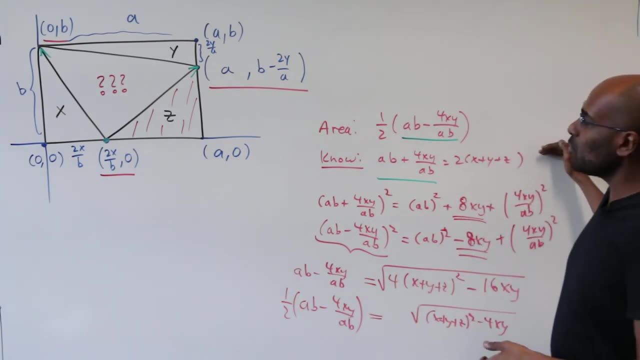 We don't know necessarily how to go about doing that, But if we coordinate things we can at least use the short shoelace formula to get an expression for the area, Together with some information that we know that we got from this last triangle. 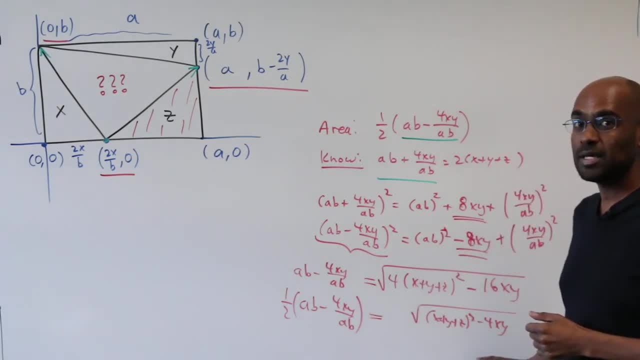 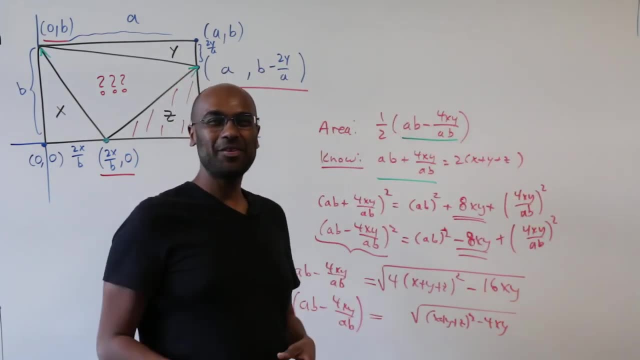 we can piece things together to figure out the quantity that we want, And we actually avoided using the quadratic formula in this particular case, So I hope you liked today's video. If you'd like to see more videos like this, subscribe to the channel. 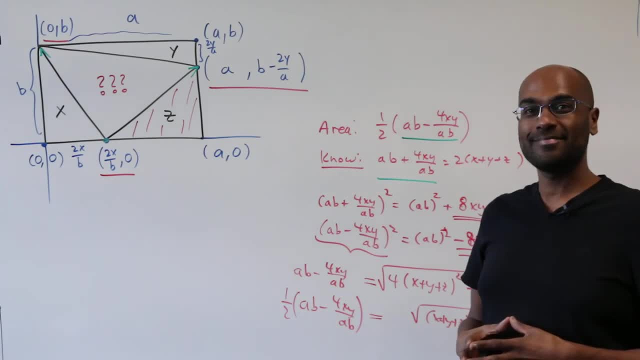 And if you'd like to get notifications, click the little button in the corner.